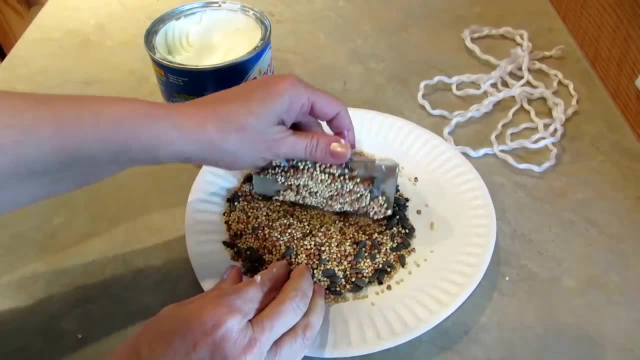 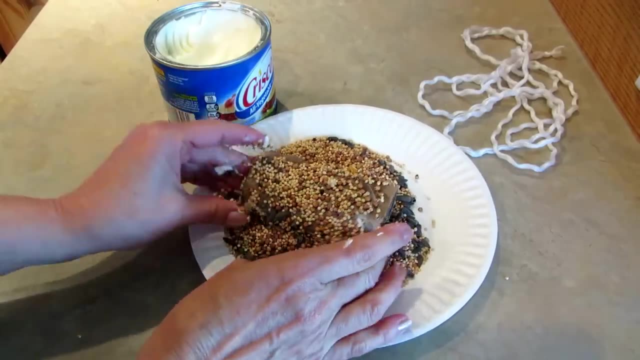 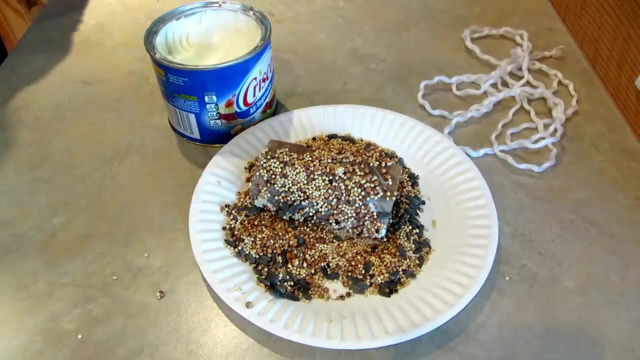 it nice and sloppy and then you just roll it in the bird seed and it's going to stick all to it. So see, the gloppier you make it, the more that will stick. Then you take any kind of string you have, thread it through and make it to whatever length you want, and 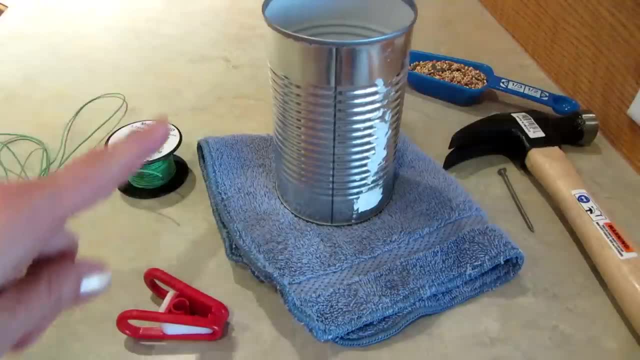 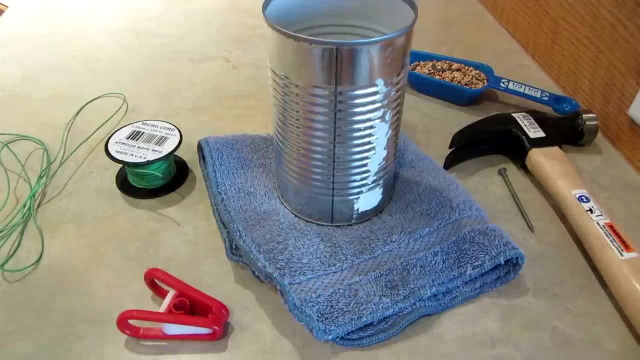 go hang it out in your tree. Well, you need an empty can, a clothes pin, some quarter string- any kind will do a hammer, a nail- and some bird seed. So the first thing you want to do is take your can and lay it on something to help it not roll around, and you 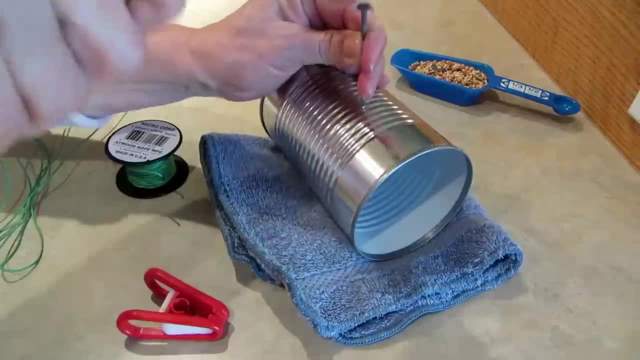 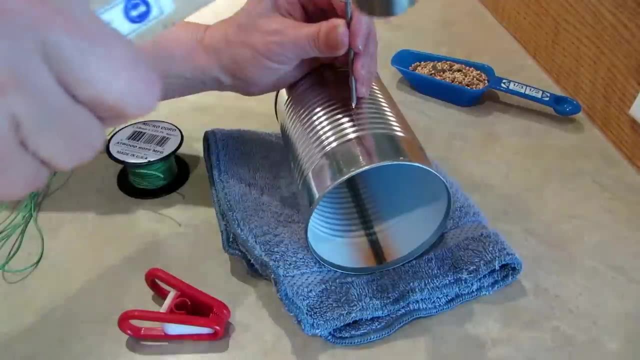 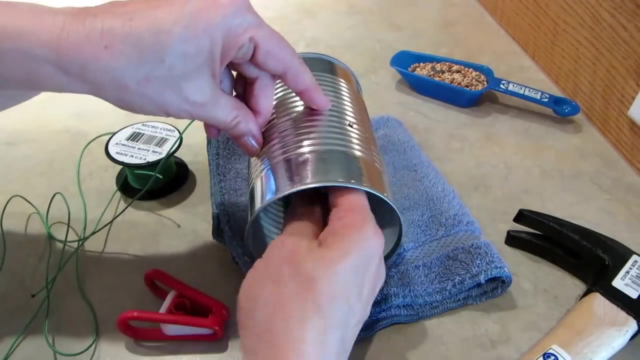 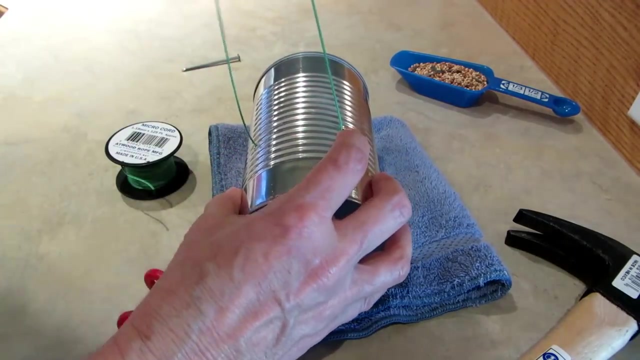 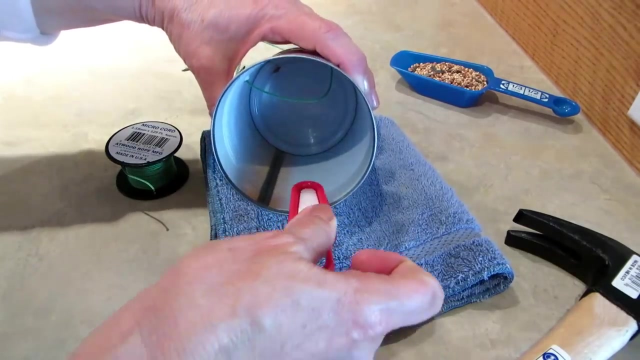 want to hammer two holes in it Now. you want to thread your string through the two holes And leave it nice and long, for however long you may want to hang it in the tree. Then you clip your clothes pin on here. Any kind of clothes pin will do. Fill it up with bird. 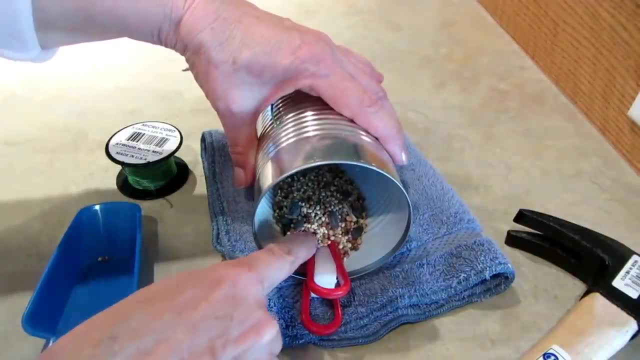 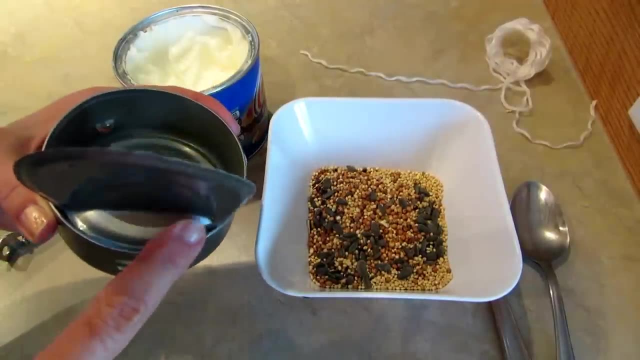 seed, Your bird can land on the clothes pin and eat away at the seed. By the time you open up a can of tuna, don't take the lid all the way off. Leave it on the lid for a few seconds. You want it to be a little bit more transparent. You can see that the 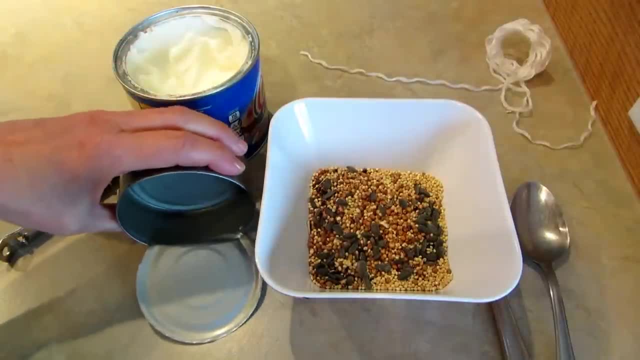 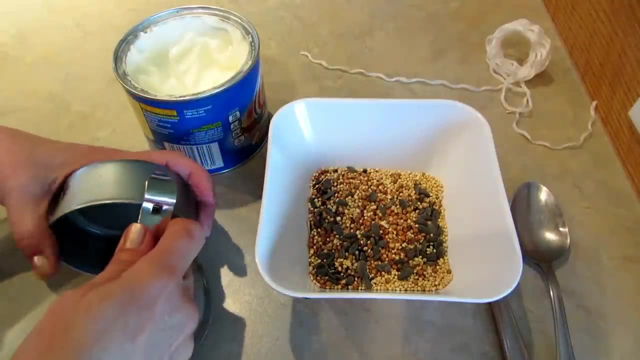 it partly attached and fold it down for a little stand. then you want to take just a church key and poke a hole in it. I poked one there, I'm going to poke another one right here and I'm going to put a string through it. realize now that. 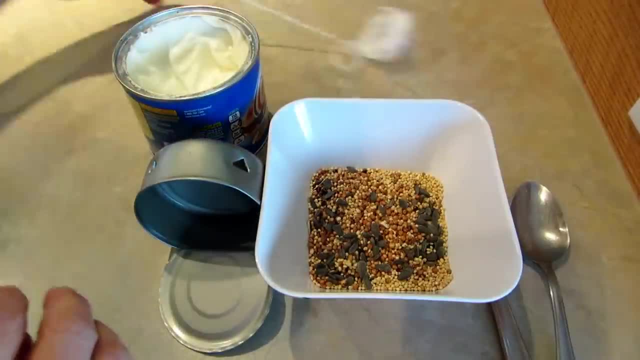 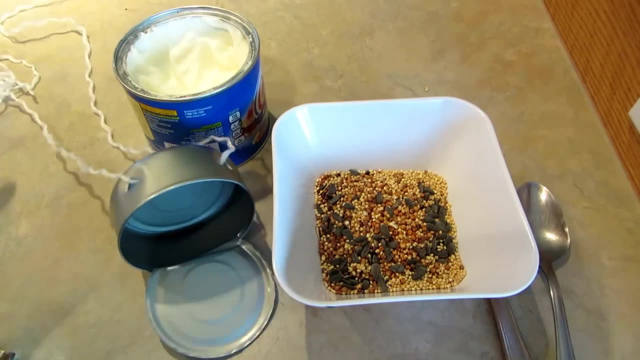 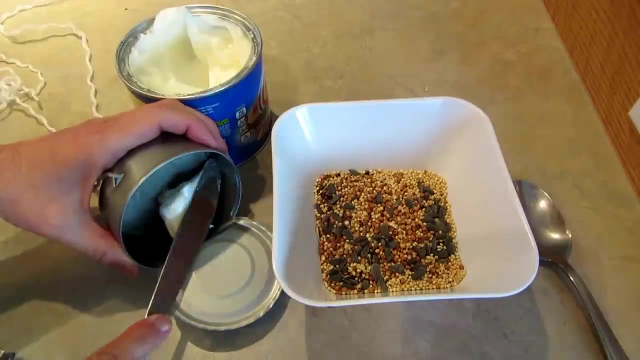 this is sharp, so you want to be very careful. so if you're doing this with little ones, you might want to push it through for them so they don't get cut on that. now you want to take a knife and get a big old scoop of Crisco, or? 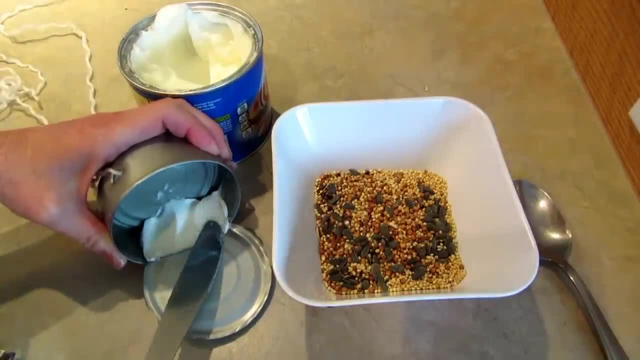 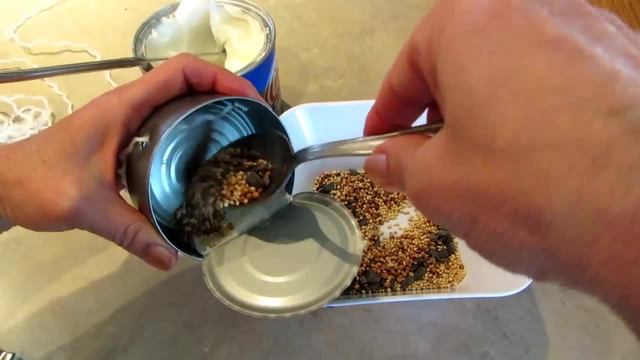 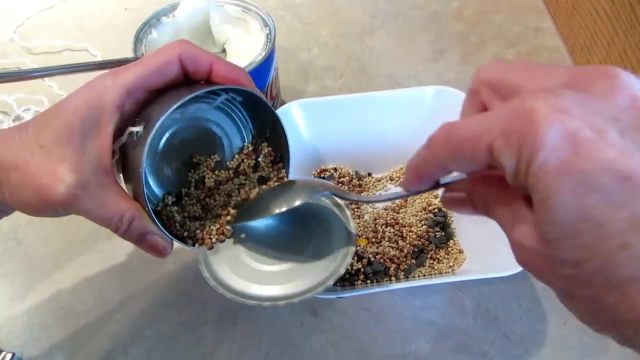 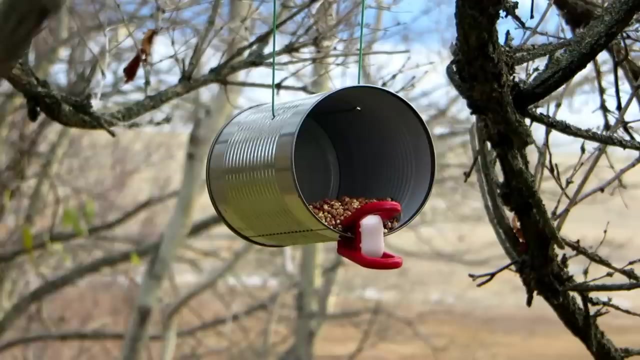 shortening and glob it right in there. now you want to take a scoop of seeds and stuff that right in on top, and the Crisco is going to help settle the seeds and hold them in there. hand up some bird feeders for your feathered friends and please subscribe to AlaskaGrannycom.